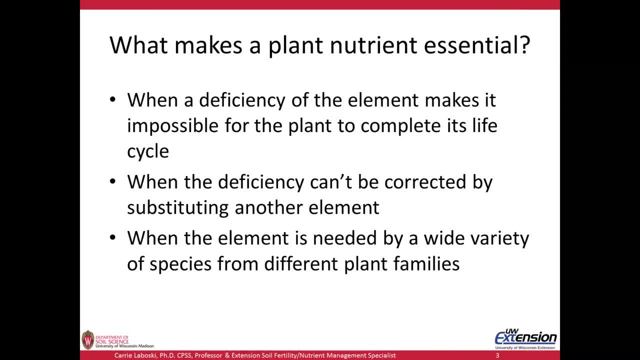 And then a little bit on cation exchange capacity. So first let's talk about what makes a plant nutrient essential. Well, there's a few criteria that would put a nutrient in the essential category. So the first is when the deficiency of that element makes it impossible for the plant to complete its life cycle. 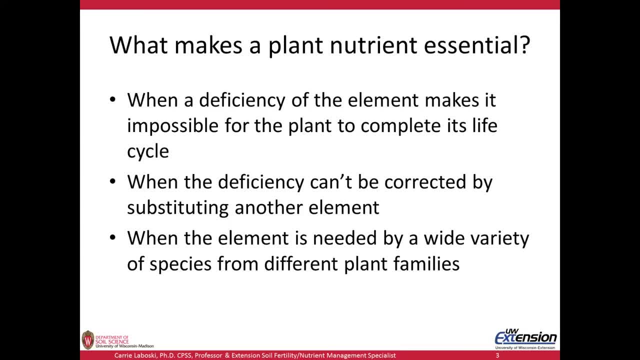 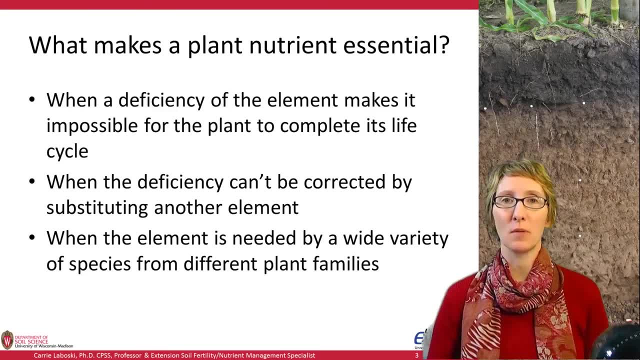 That's pretty clear cut. Another one is when the deficiency can't be corrected by substituting another element. It's obligate that you need to have that particular nutrient. And then third is when the element is needed by a wide variety of species from different plant families. 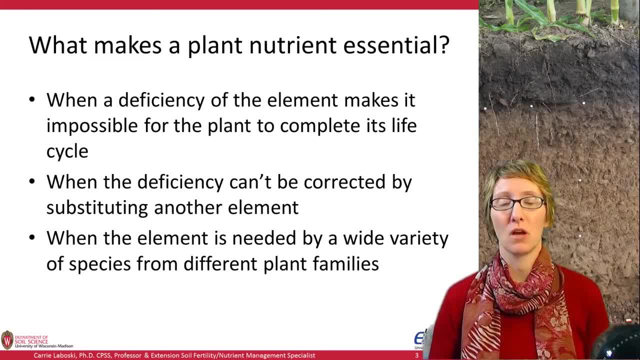 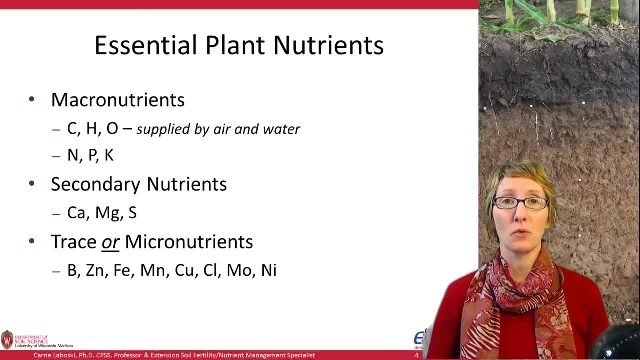 That suggests that it is very important overall for the plant kingdom. Now our essential plant nutrients. just to go through them real quickly. we'll have more in depth on these in other videos. We need to think about our macronutrients. 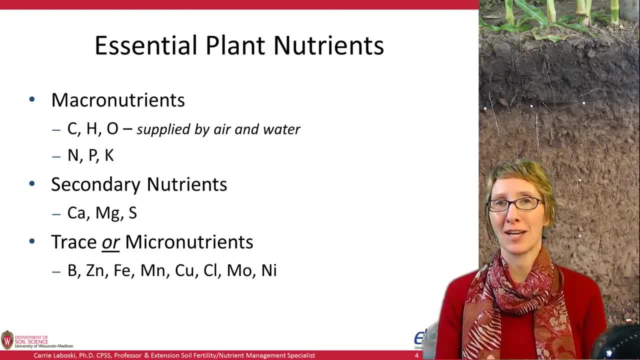 And sometimes we don't really think about carbon hydrogen and oxygen as macronutrients, Mainly because they're supplied by the air and water. They're not really, you know, we're not applying them in fertilizer, But we have to keep in mind that they are used in large quantities by the plant. 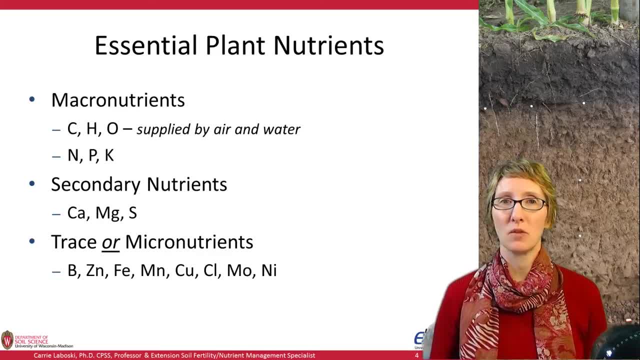 So they truly are macronutrients. Then we get into nitrogen, phosphorus and potassium, Again used in large quantities. Secondary nutrients are considered secondary because they're required by the plant, but in smaller amounts than the macronutrients. 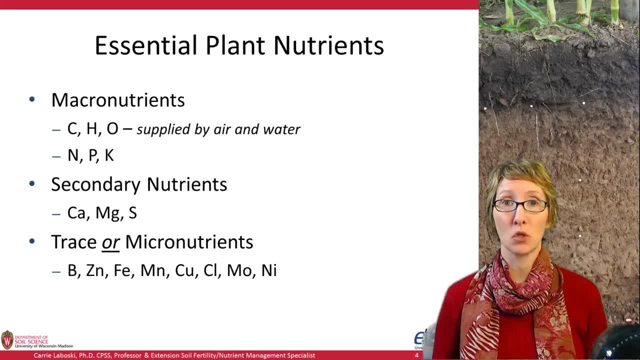 And the secondary nutrients include calcium magnesium and sulfur, And then we get into the micronutrients, or sometimes they're called trace elements. Now, these are nutrients that are required in relatively small quantities, And there's a whole host of them here. 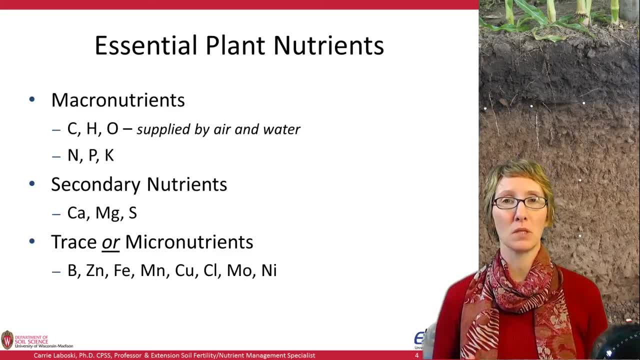 Boron, zinc, iron, manganese, copper, chloride, molybdenum and nickel. Now we need to keep in mind that, whether we're talking about a micronutrient or a macronutrient or anything in between, 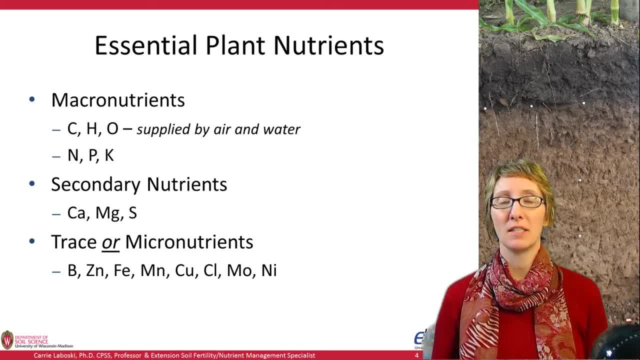 that different plant species have different requirements. Some plants have a greater need for potassium than other plants, And then, when we get into the micronutrients as well, some have higher requirements than others, And that's what makes each individual crop different and unique. 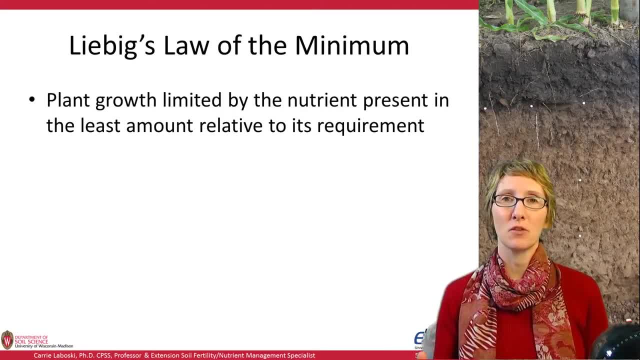 Now, before we get too far along, I think it's important to keep in mind what Liebig's Law of the Minimum is, And this relates to plant nutrients and their essentialness- And what it is is when we think about nutrients and limiting nutrients. is that the plant growth will be limited by the nutrient present in the least amount relative to its requirement. So you could have a piece of ground that's both phosphorus and potassium deficient, but maybe you only really are observing potassium deficiency. You're not really seeing P deficiency symptoms. Maybe you're applying P fertilizer and you're not getting a yield response to it, even though soil test might be low. What's happening there is that the K is so deficient that it doesn't matter what you're doing with phosphorus to try and give the plant more. 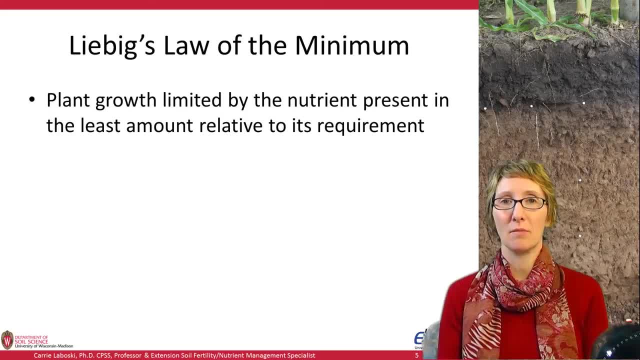 We need to get the K built up and into the plant in a greater quantity before the phosphorus could become limiting. So it's just important to keep in mind that it's not just looking at one nutrient alone. We need to look at them in the complex nature that exists relative to each other. 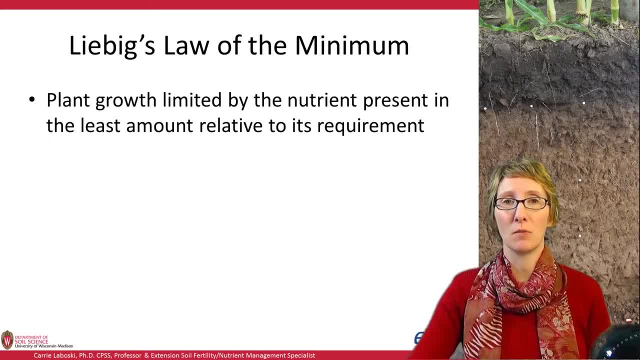 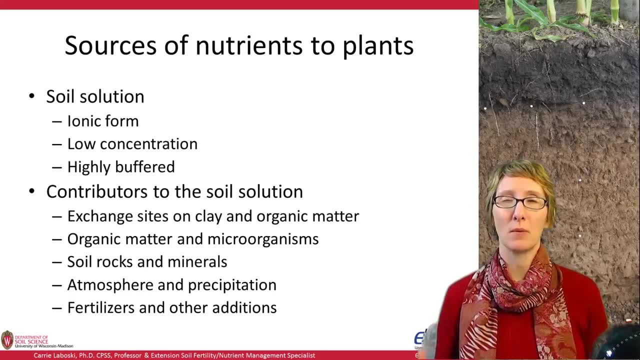 and to the total requirement of the plant. So now when we start thinking about sources of nutrients to plant, we can think about from fertilizers and manure sources like that, but when we get down into the soil a little bit more, where plants get their nutrients, 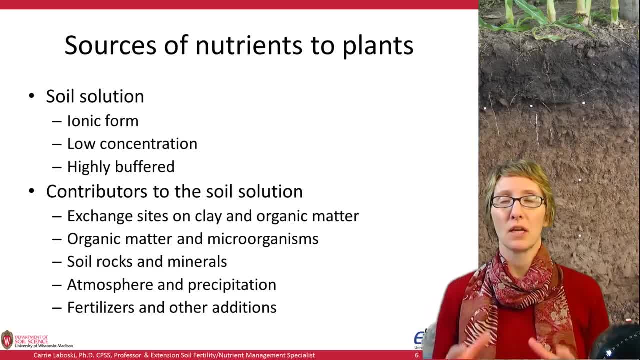 From the soil solution is one Within the soil solution, that's the water that exists in the soil. Very simply, that The nutrients in the soil, like that, are in ionic form. The concentrations tend to be very low. Now, granted, when you apply fertilizer. 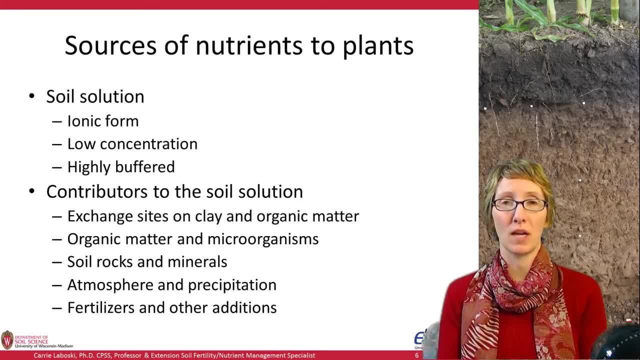 right next to a granule. the concentration might be quite high for a period of time, but it diffuses outward And the nutrients in the soil solution tend to be fairly buffered, meaning that, as the plant will use the nutrient from the soil solution, 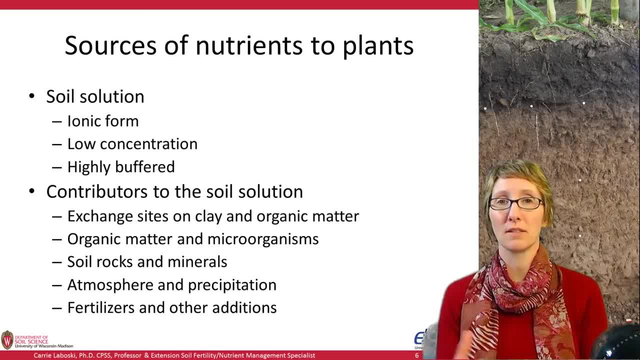 it will become available from other pools like, say, the cation exchange capacity and ability of the plant to use those nutrients. Now, some of our contributors to soil solution. Okay, this is the whole host of where nutrients are in the soil and how they're held in the soil. 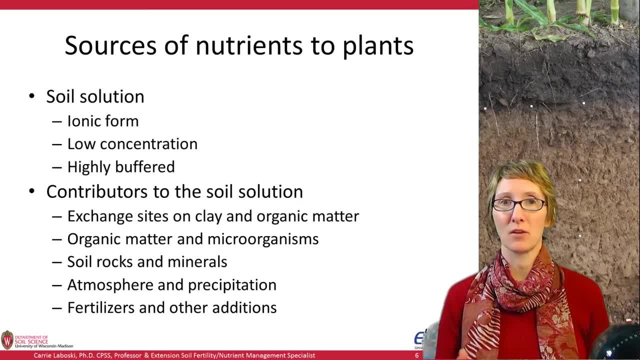 So this we're looking at: cation exchange capacity. Okay, so that would be our exchange sites on clay and organic matter. When we think about organic matter itself, as it mineralizes, nutrients are released from organic matter And microorganisms mediate that mineralization process. 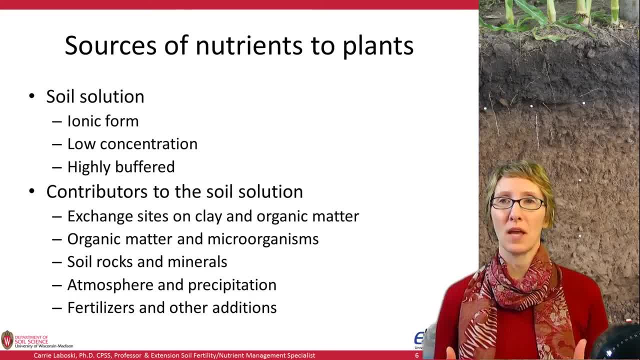 and release of organic nutrients. We also have release of nutrients. as the soil weathers, You know, as rocks and minerals weather, some nutrients are released. When we think about atmospheric deposition of sulfur and precipitation, you could have some nutrients precipitating or atmospheric deposition. 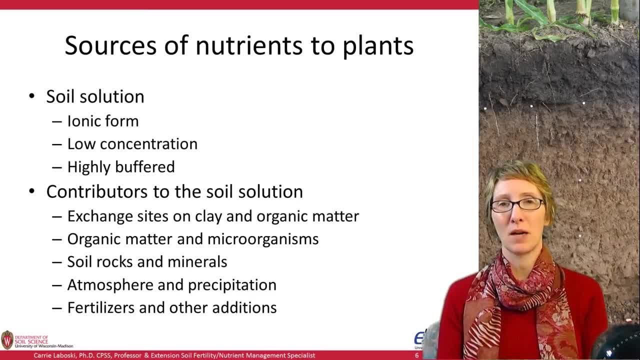 In some ways, they may be byproducts of air pollution, which sulfur is in some cases, but it's nonetheless a manner in which nutrients are placed into the soil, And then, of course, as we already mentioned, fertilizers and manure and other additions, waste products, etc. 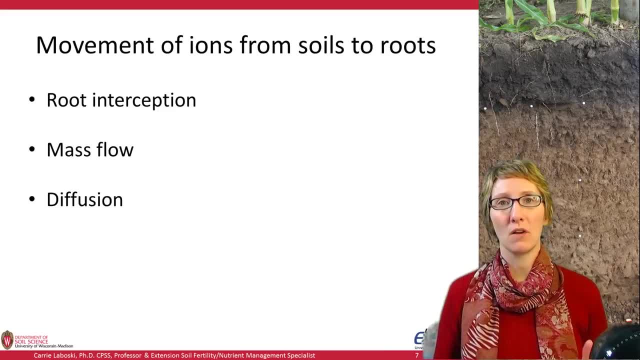 Now I want to spend a little time talking about the movement of ions from soils to roots. Okay, Because this is really important And not every plant nutrient behaves the same way, So there's three key ways that nutrients move to the root. 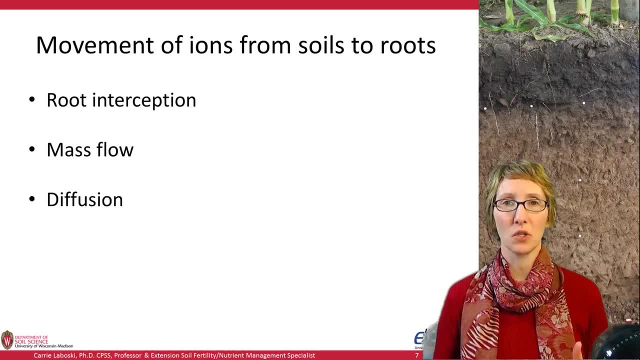 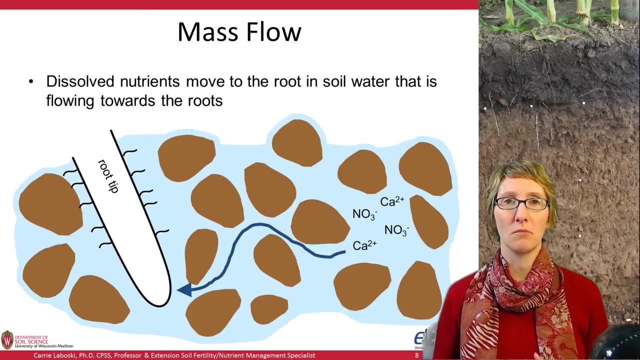 Okay, The first one is root interception, then mass flow and finally diffusion. So now, in the next few slides, as we talk about these different methods of nutrient movement to the root, I have a little cartoon that I've drawn so that you can have a better understanding of what's happening. 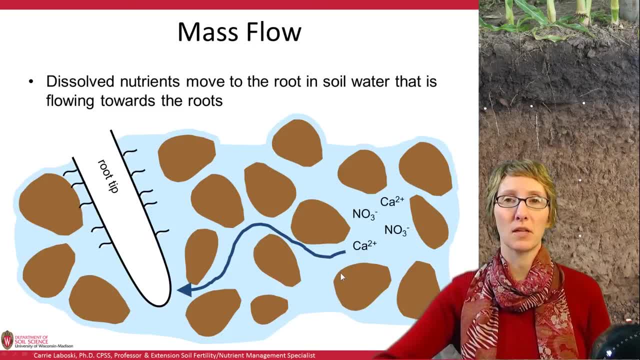 And so we'll just go over the cartoon a little bit, because you'll see it a couple times. So here we have our root tip right here, And these are the root hairs. extending out from the root tip, We have the soil particles. 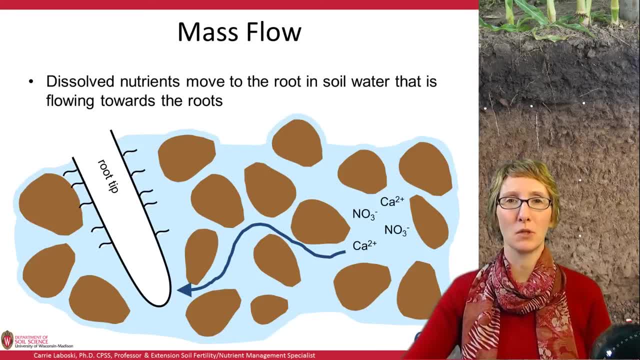 Okay, And I have them kind of spaced big. I'm, you know, looking at a high-powered microscope here, So they're kind of spaced a little far apart, And the blue here represents the soil solution, So we can see where the nutrients are held on the soil. 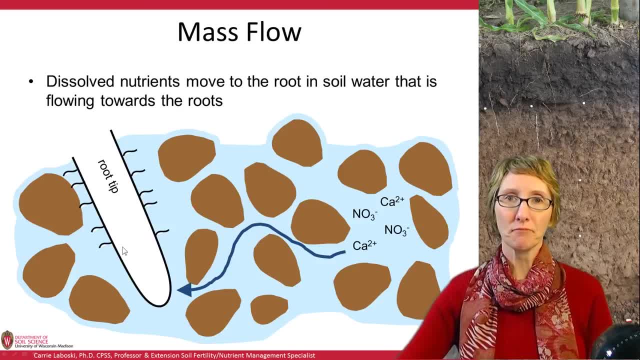 they're in the soil solution and how they're getting to the root. So now to specifically look at mass flow here. this is where dissolved nutrients are in the soil solution. Okay, So here we've got calcium and nitrate. They're dissolved. 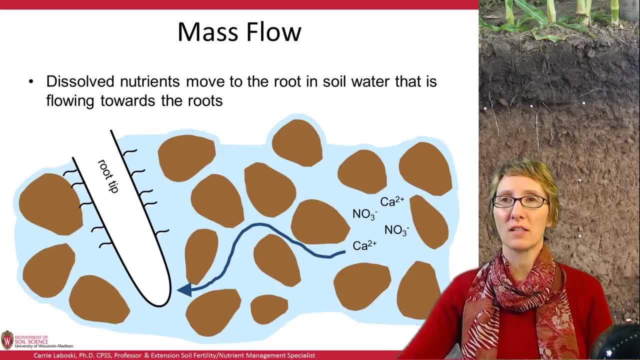 They're in the solution And they move in water as it's flowing to the root. Okay, So that root is here, Okay, It is taking up water. The plant needs water And so, as it's using water and water is flowing towards the root tip, 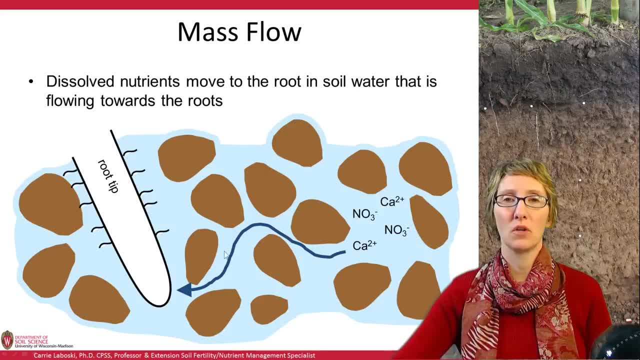 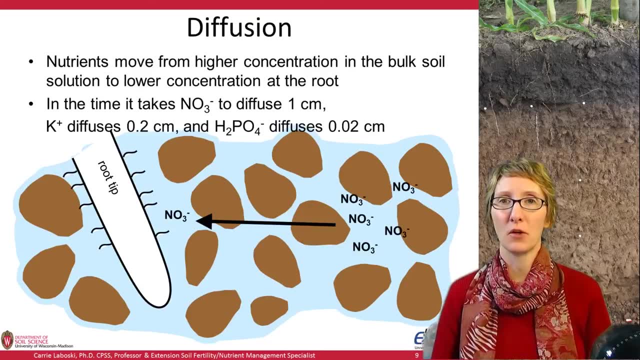 all these nutrients here. they're just kind of moving all along with that flow path of water. It's just mass flow. Now diffusion is another method, And this is a term you may remember from high school chemistry class. It's simply the movement of nutrients, or anything. 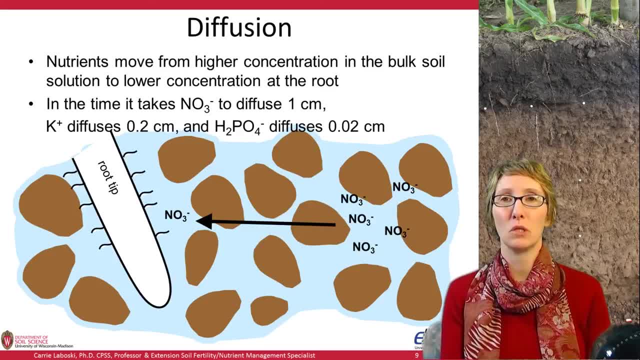 if you're just talking about basic diffusion from higher concentration to lower concentration. And here's an example with nitrate. We've got a high concentration of nitrate out in the bulk soil solution And we've got a low concentration of nitrate by the root tip. 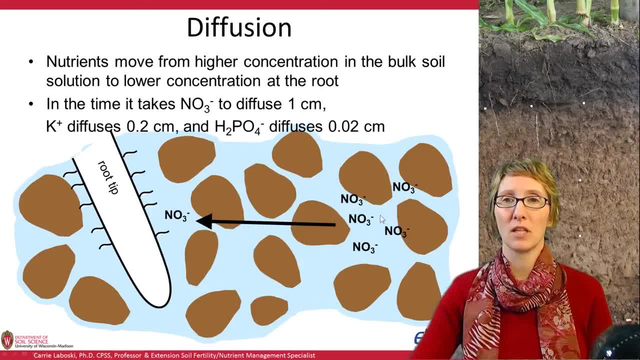 because the plant's using it, So it's taking up, So there's not much here, There's a lot over here, So it diffuses across. Now diffusion is not as fast of a process And, to give you some idea of timeframes, 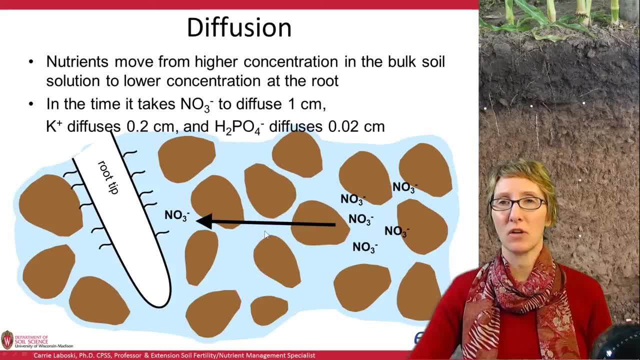 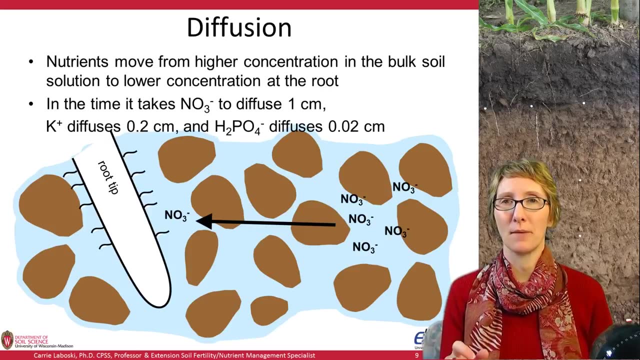 we have timeframes involved here. In the time that it takes nitrate, for this example here, to diffuse one centimeter, potassium will diffuse .2 centimeters and phosphate will diffuse .02 centimeters. That's in that same amount of time. 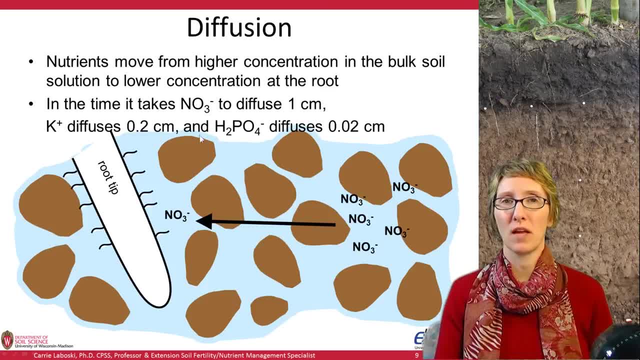 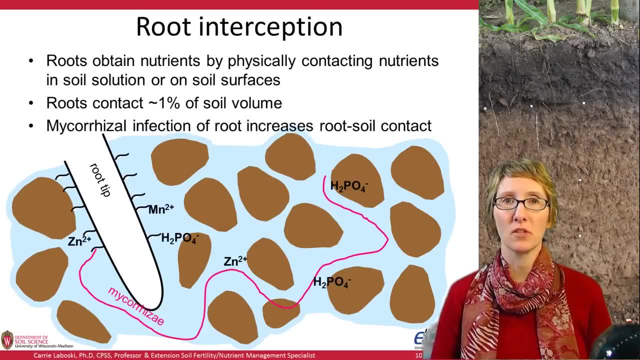 So you can see that nitrate's going to diffuse much faster than potassium or phosphate. And our third mechanism is root interception, And this is where roots need to physically contact the nutrient in order to be able to start taking it up. It's not going to move by mass flow or diffusion very much. 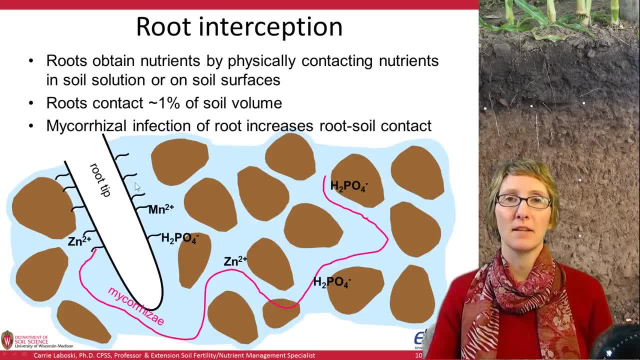 It would be very small amounts, And what's important with this is that roots generally can be thought to only explore about 1% of the soil volume, And that 1% is not very much So if a plant has to rely on root interception. 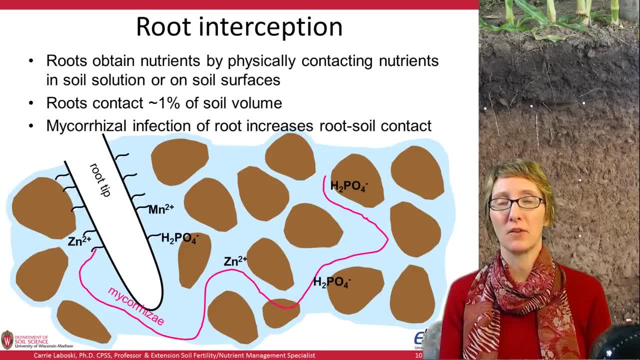 to take up a nutrient. they're not exploring much soil, So it's going to be a little bit harder for the plant to get that nutrient- Many of our micronutrients, like manganese and zinc. the plant relies on root interception to obtain those nutrients. 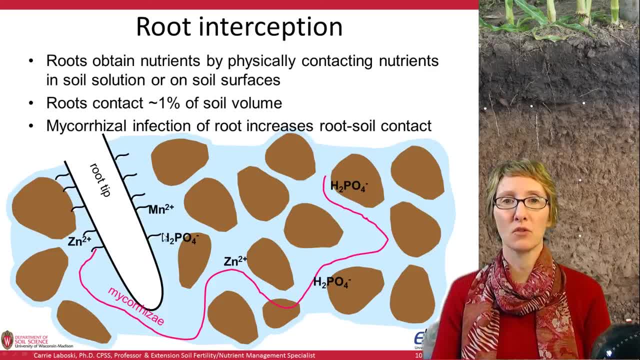 Phosphate is another one. Now, here I have also drawn in this pink color, is a mycorrhizae. So remember this is a fungus that infects the roots. This is the root tip And what happens here. so it's actually infecting a root hair. 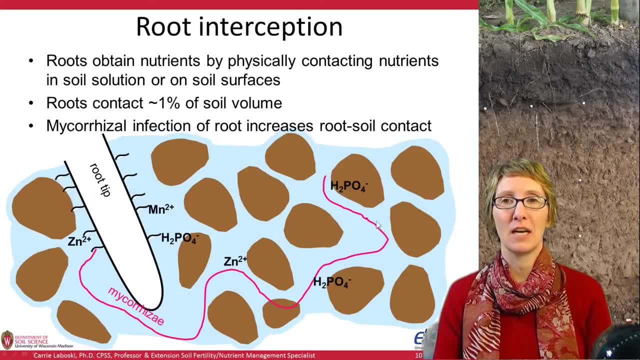 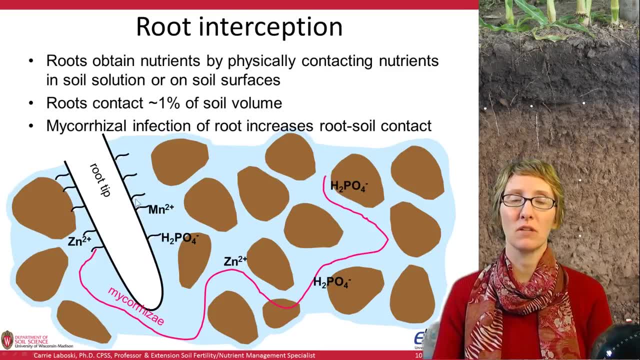 as I have it drawn, and it effectively extends the area or the volume of soil that the root is exploring, Because now this phosphate over here is really far away from that root tip, But if we see where that mycorrhizae is growing, 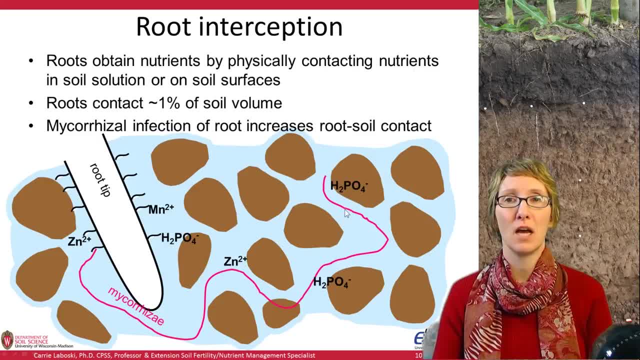 it's right around that phosphate, So the phosphate can be taken into the mycorrhizal structure and then ultimately move back to the root tip, And so that's a nice relationship between roots and mycorrhizae. The mycorrhizae help the plant. 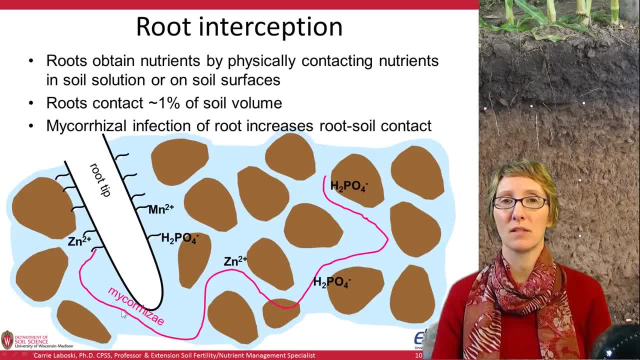 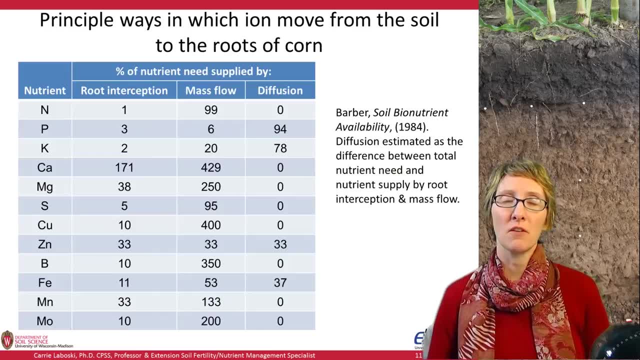 take up some of these nutrients and then the plant provides some carbohydrates to the mycorrhizae so that they can live. So just to give you a feel for how important these different mechanisms for nutrient movement are, we have this chart that shows the principal ways. 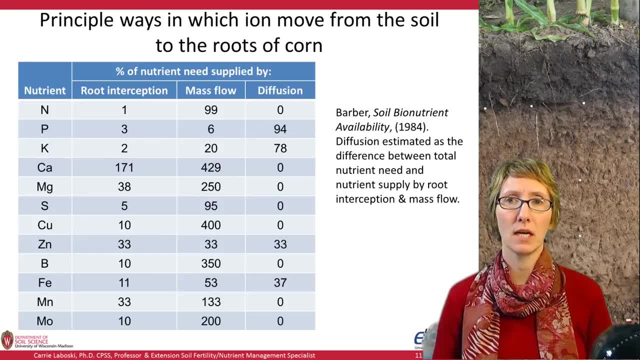 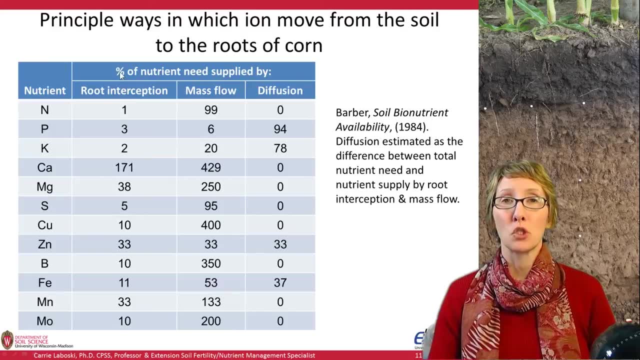 that plants move from the soil to the roots of corn, And so we have our different nutrients here, and we need to keep in mind what we're looking at, And here it's the percentage of nutrient need which is supplied by the different mechanisms. 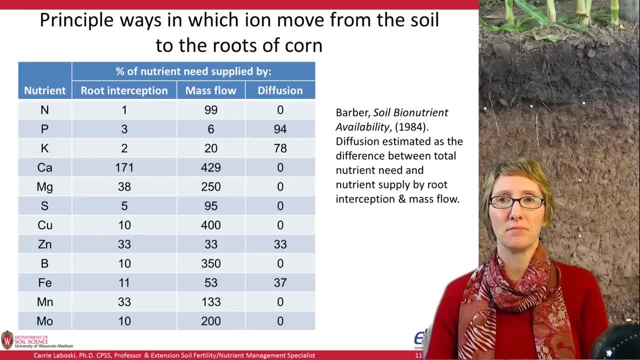 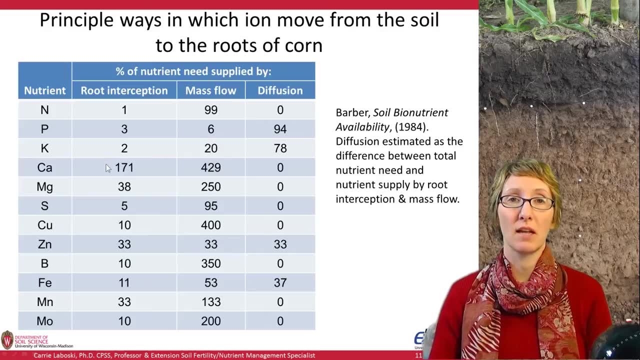 So if we look at root interception we can see that calcium we can get 171% of nutrient needs supplied by root interception. That doesn't necessarily mean that's taking up all that it could, But it's saying that root interception could supply that much of the nutrient need. 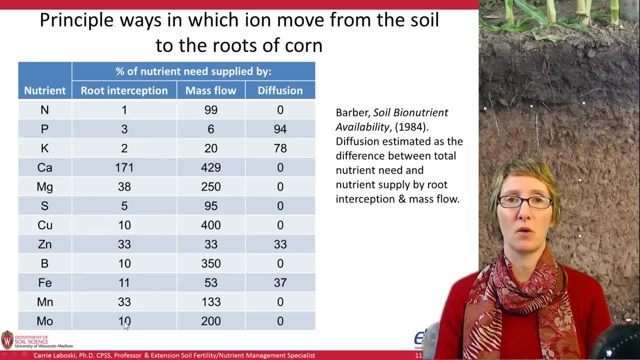 And then you can see that there's a range for the different nutrients of how important that is. Then we look at mass flow And you can see there's a large amount or a large percentage of the plant nutrient need can be supplied by mass flow. 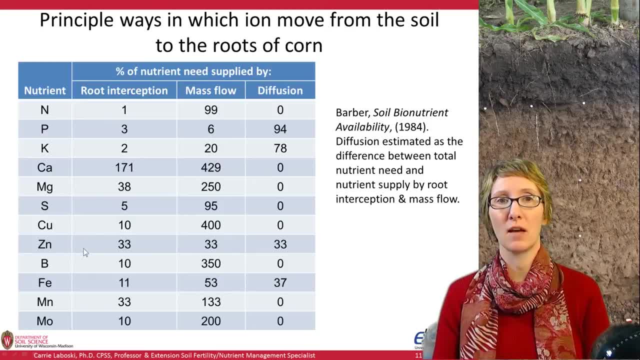 But it can vary. So if we look at manganese, that drops down to 33%. That's not a lot Iron. another one, another micronutrient, smaller amounts: Phosphorus: only 6%, So a pretty small amount. 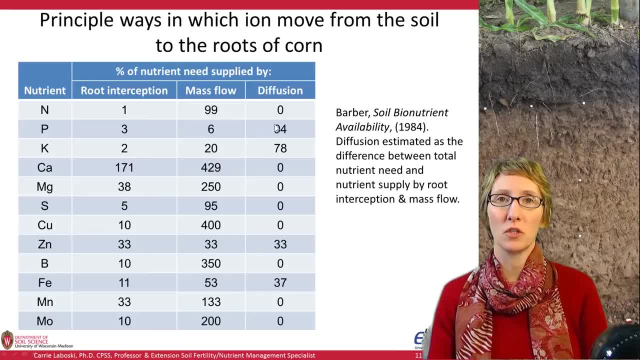 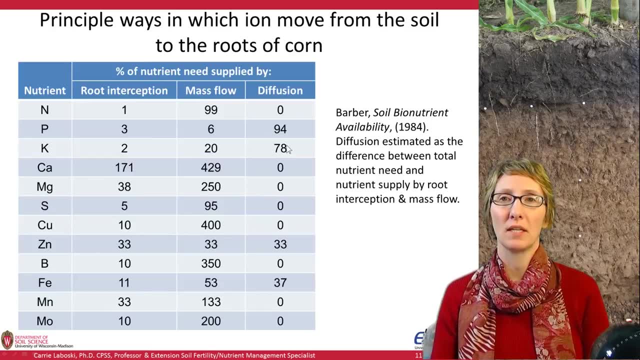 Now diffusion. how they determine the amount of nutrient need supplied by diffusion is they simply took the difference between the total nutrient need and the nutrient supply by root interception and mass flow. So some of these have zeros because root interception and mass flow can supply everything. 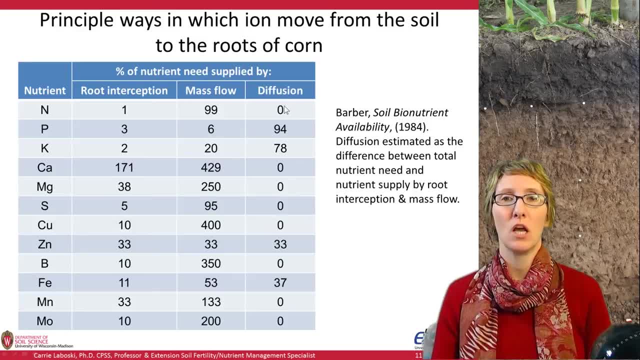 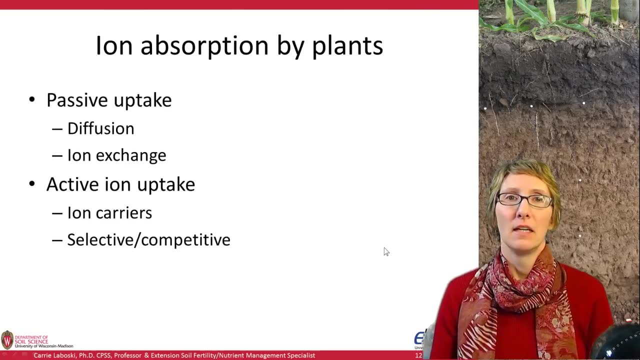 Therefore, diffusion is not needed and is probably inconsequential. But you can see that for several nutrients diffusion is extremely important: P and K very important. Zinc and iron, because we're not doing it all with root interception or mass flow. Now, when we think about 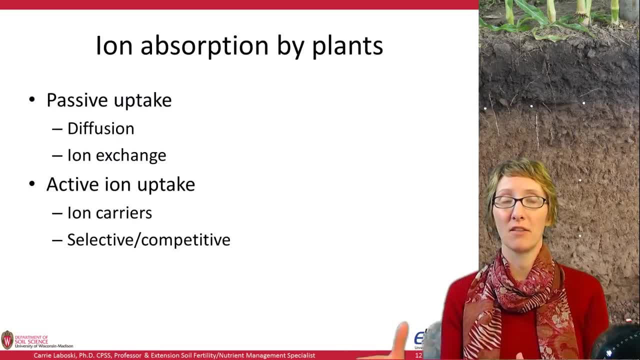 plants taking up nutrients. there's the matter of getting the nutrient to the root tip, which we just talked about, Getting the nutrients into the plant. So we have different means and we call them passive or active uptake. Now in passive uptake is where 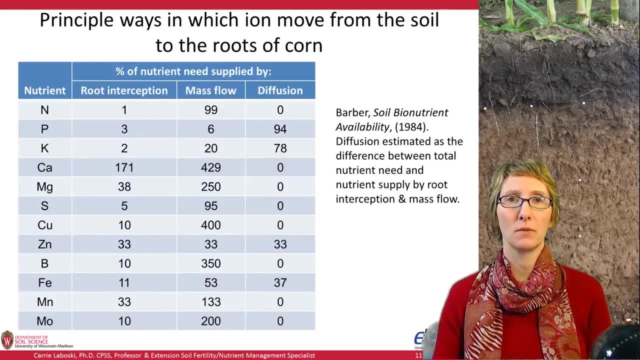 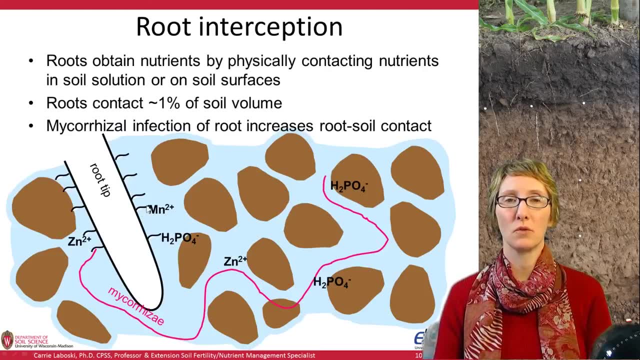 you have a nutrient and we're just going to go back one slide here, two slides. So in passive uptake you have a nutrient that has made it over to the root tip And we can have diffusion from outside of the root into the root. 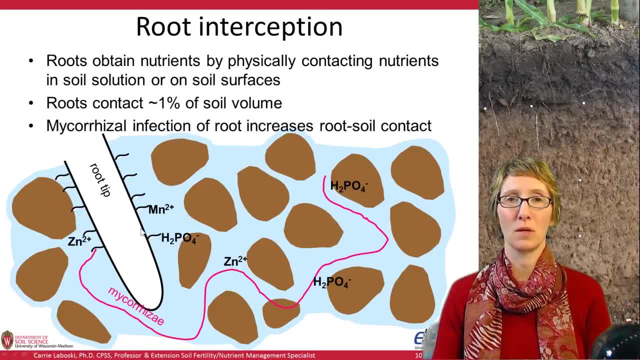 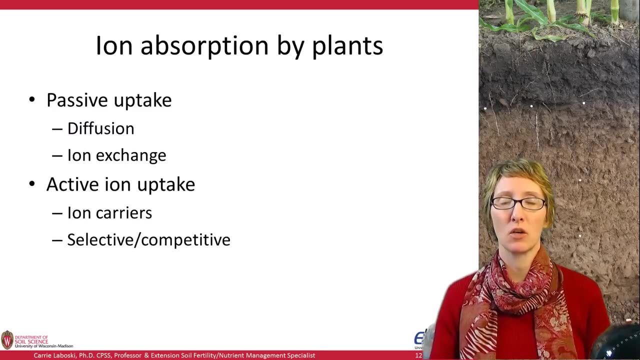 So that might be a little confusing because you could have diffusion across the soil. but for active uptake you could have diffusion across the root membranes into the root. Then you can also have ion exchange. So the root tip is going to release, say, 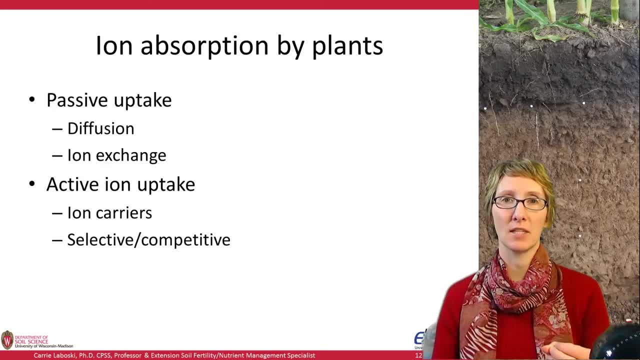 a hydrogen ion, and then it maybe takes up a potassium ion, because it's maintaining electrical reality, releasing one positive charge, taking up a positive charge, Just simple ion exchange actions. Then we have what we call active ion uptake, And this gets a little more interesting. 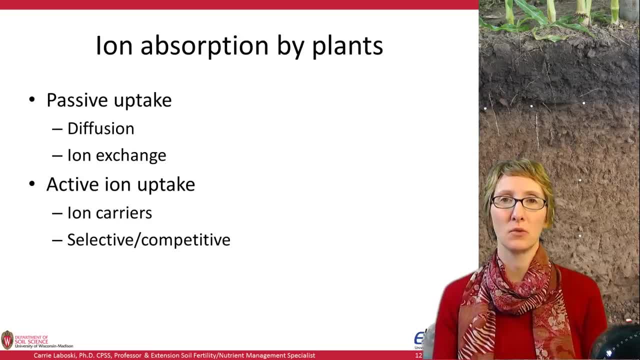 because it requires the plant actually do something to get the nutrient. It's just not happening by itself. So there are specific ion carriers and they can be selective or competitive, And they actually are within the cell walls of the root And so not everything is. 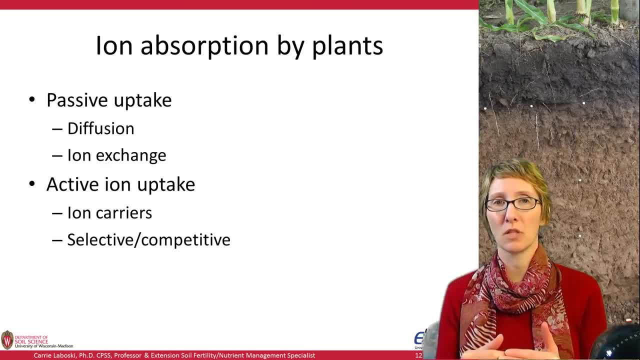 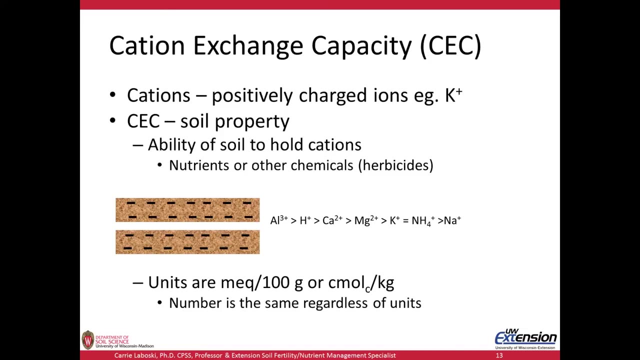 going to penetrate into that root cell wall. So there's actual active uptake, meaning the plant has to expend some energy to get those nutrients into the plant. Next we'll move on to cation exchange capacity. Cations are positively charged ions, For example potassium. 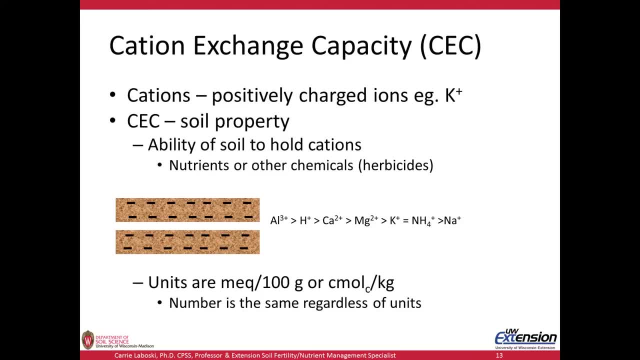 Hydrogen calcium. they're all positively charged. Now, the cation exchange capacity is a property of the soil. It's a basic way to think about it. It's the soil's ability to hold cations- Pretty simple. Now these cations can be nutrients. 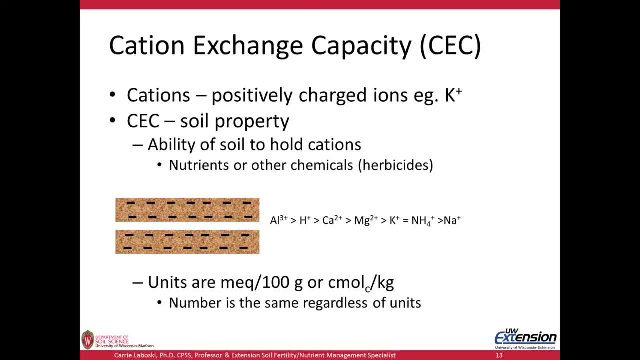 That's what we typically think about, But we also have to keep in mind that other chemicals might be cations as well, For example herbicides. Now, this little diagram here is showing some clay layers in the soil, And the black represents our negative charge. 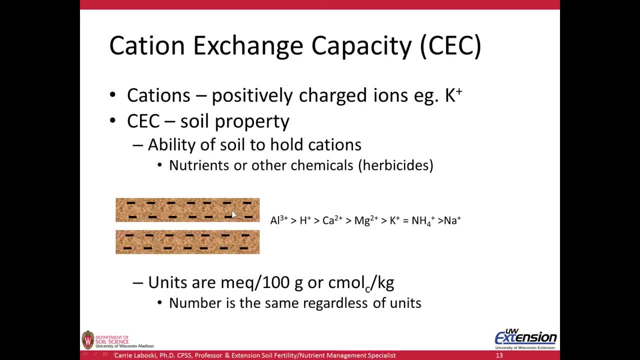 So the clays themselves, after the process of isomorphic substitution, develop negative charges, And that's what's showing up here with the black. And because they have a net negative charge to them, cations will be held onto the surface of the clay. 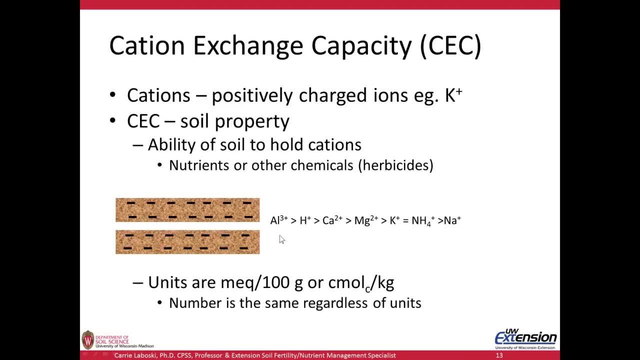 Now here I have a series of cations listed in the order of over. here on the left, with aluminum is greatest ability to be held onto the cation exchange and that has a plus three. Typically, the higher the charge, you're going to have a little better. 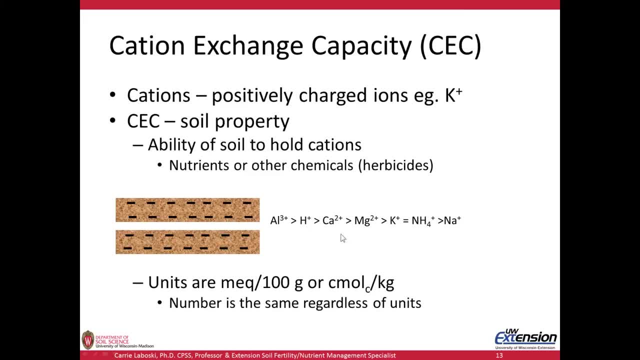 binding onto that cation exchange. so that's why we have aluminum at the top and calcium and magnesium higher up. Then we get into the single positive charges: hydrogen, potassium, ammonium. Those are a little bit different in their order and they're related to. 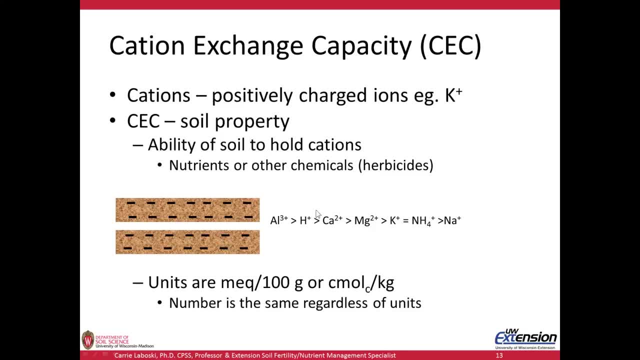 the hydrated radius. So if you have something that's small like a hydrated radius like hydrogen, that's got some ability to kind of wiggle in there and be held on the cation exchange, compared to something that has a large hydrated radius, that's kind of big. 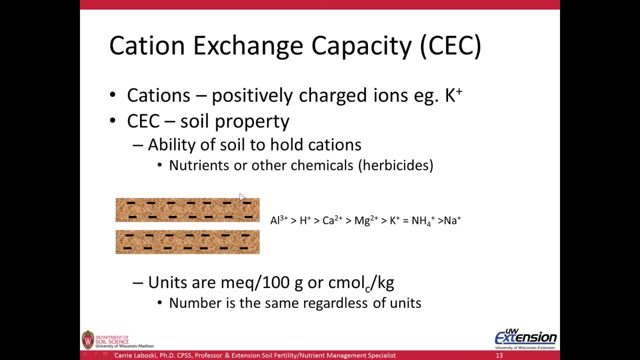 and fat and a little bit harder for it to be held with as much static electrical charge attraction between the two of them Now with cation exchange capacity. the one thing that can be confusing for some people are the units. Now you may see units of milliequivalents per hundred grams. 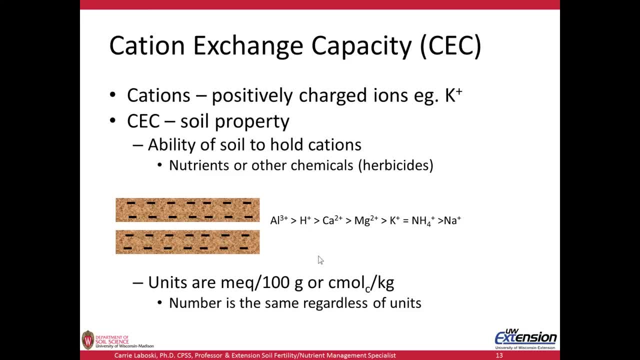 that's sort of an old fashioned term of units, but it still gets some use today. and then you have the more modern sort of metric or international set of units. that's called centimoles of charge per kilogram. And the nice thing about the units on cation exchange is that 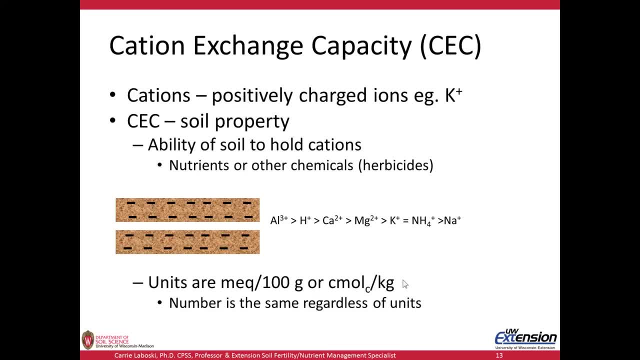 you don't have to convert one to the other the same thing. So if you have five milliequivalents per hundred grams, you have five centimoles of charge per kilogram. So that's really handy. So you don't have to worry about the units too much. 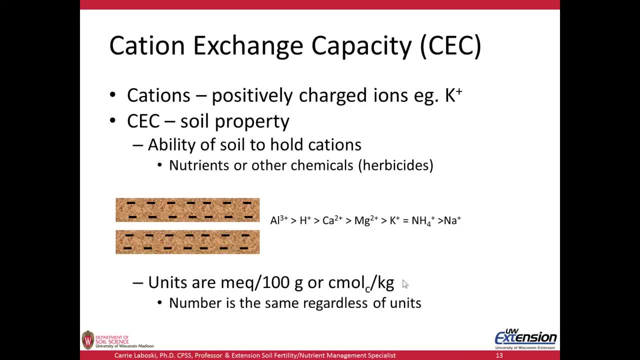 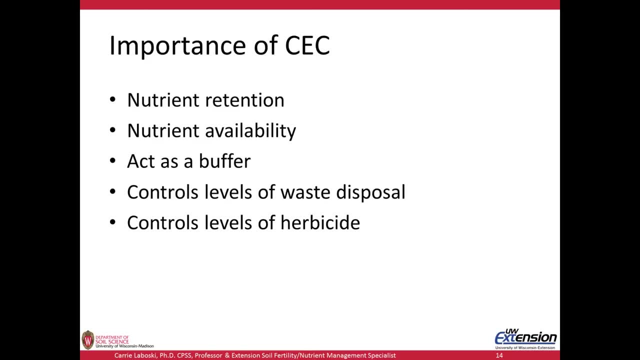 because the number's the same, and this is one of the very few places where you're going to see something that simple that you don't have to convert units. Now we need to think about the importance of the soils cation exchange, because it is a very important. 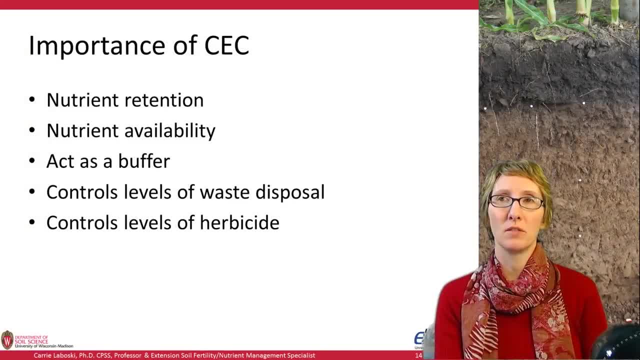 property. It helps with nutrient retention, as we just talked about Also nutrient availability in the soil, because if we can retain, if we have a soil with higher cation exchange capacity, we can retain more potassium, but that's also allows it to be able to be. 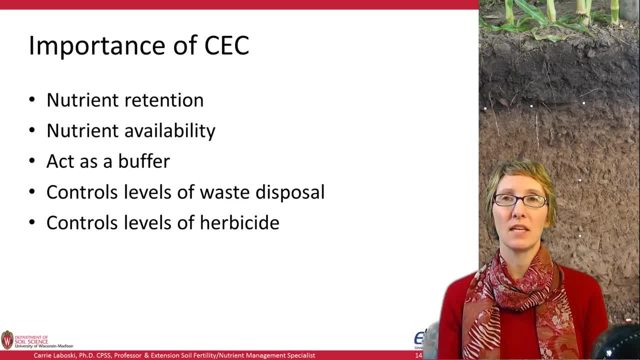 released into the soil solution. The cation exchange capacity can act as a buffer for nutrients, but remember, it can also be a buffer for soil acidity And we'll talk more about that when we get into the liming section And the cation exchange. 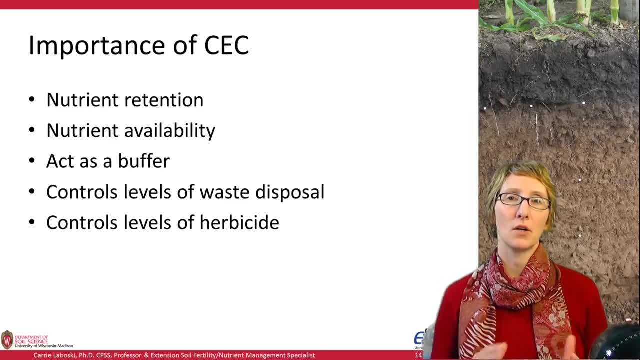 capacity can control the levels of herbicide that you could apply or that are going to be bound up to the soil and their efficacy. And then also when we think about some waste disposal, say application of food plant or food processing type waste. some of those are: 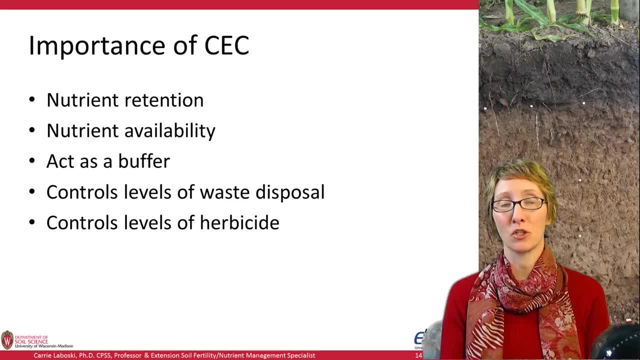 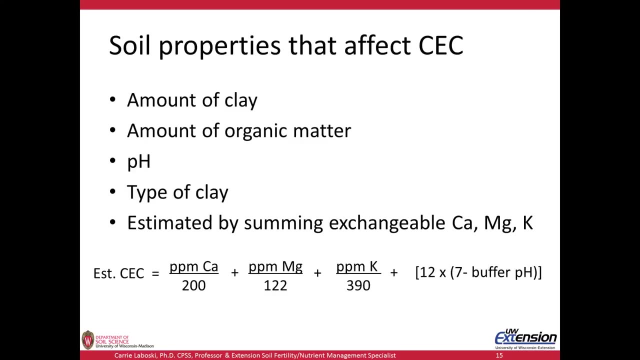 determine the amount that can be applied based on the soil's cation exchange capacity. How much can it hold of a nutrient or material? and then that's the limit for that. Now there are several soil properties that affect cation exchange capacity. First is the amount of clay. 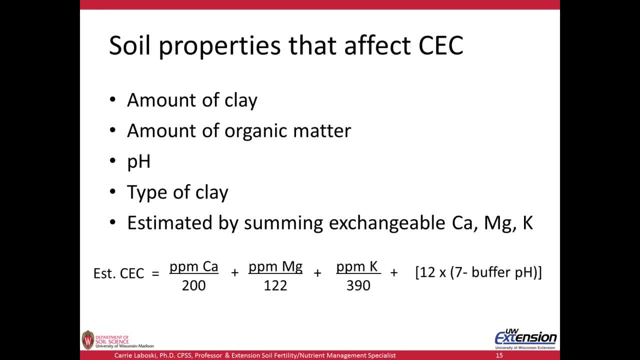 and the amount of organic matter. They all contribute to negative charges that will hold cations. Soil pH is important. The types of clay are also important. For example, if we take kaolinites versus montmorillonites, they're going to have some different cation exchange capacities. 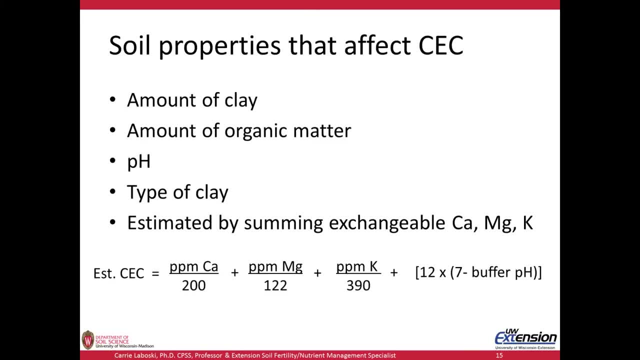 And then one thing that you might be interested in doing is estimating your cation exchange capacity, And you can do that using the little equation here at the bottom. Here you take your soil test: calcium, magnesium and potassium. Now this is where the cations have been extracted. 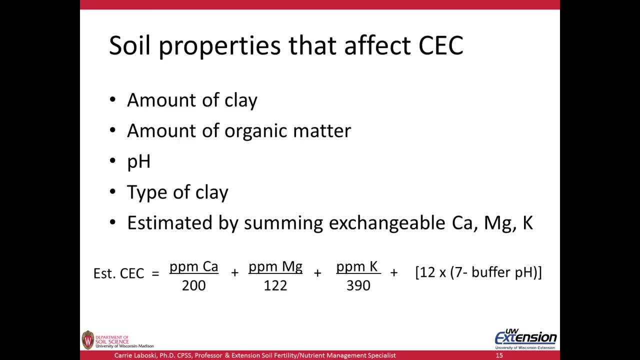 using ammonium acetate- not our typical Bray extraction that we use in Wisconsin for K, but ammonium acetate- And you take that soil test value and you divide the calcium by 200,, magnesium by 122, and potassium by 390. 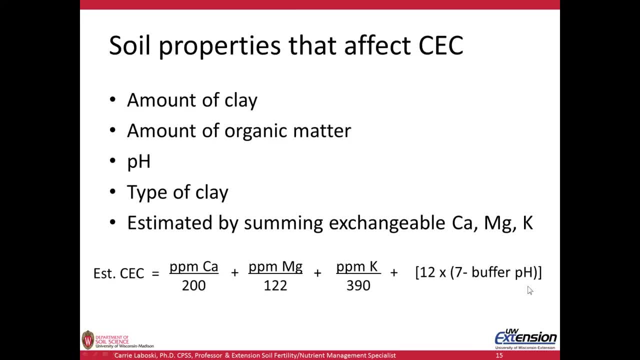 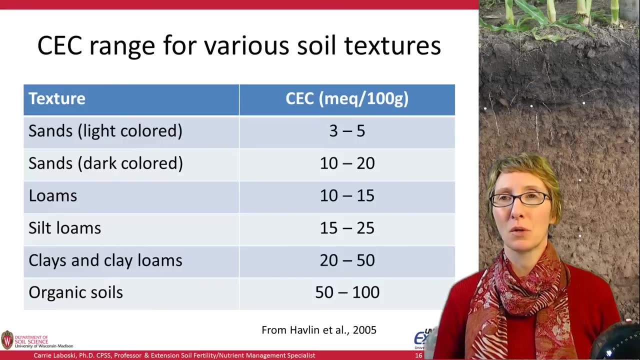 We also factor in the acidity and we do that using the buffer pH of the soil. So that's just one way you can make a bit of an estimate. It's important to keep in mind to have an idea of what are typical ranges in cation. 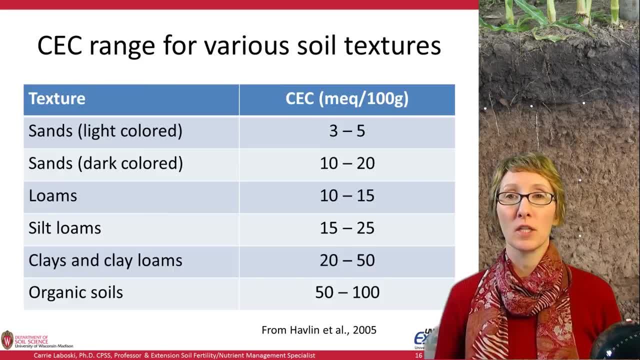 exchange capacity for different soils And this chart does a good example of showing that. Here we have at the top sands light colored, meaning that they would have lower organic matter levels. They can have a cation exchange of 3 to 5, pretty low number. 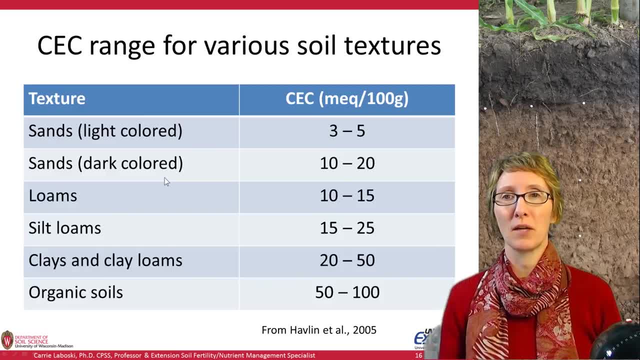 You get a dark colored sand, so it's getting a little bit more organic matter, And now you're moving into 10 to 20 tons per 100 grams, so it's really bumping it up, And the higher the number obviously is going to be related more to: 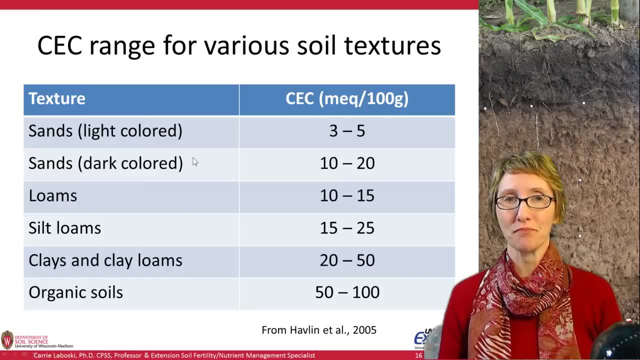 the amount of organic matter. when we're talking about these sandier soils, We look at our loams and silt loams, clays, clay loams. so all these soils, as we get, as we're going down in this table, we're increasing the clay content. 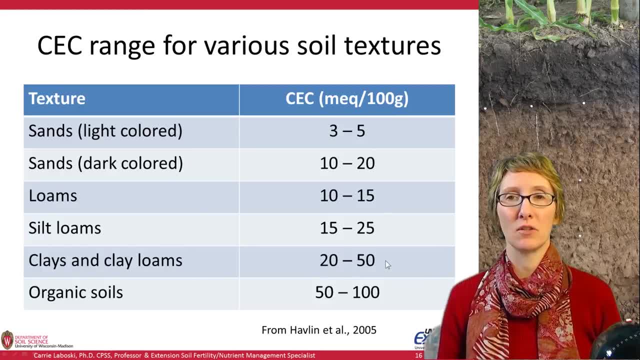 to this point And you can see the cation exchange content is a direct increase. And then we have organic soils, mucky type soils, that's what we're talking about. they can have very high cation exchange. So just have an idea. 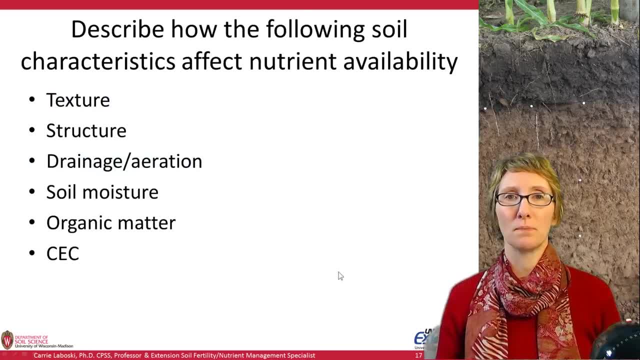 of what you might expect for cation exchange based on texture alone. Now, as you're preparing for your CCA exam, one of the things you should be able to do is know and be able to describe how different soil characteristics affect nutrient availability, And we're not going to go into depth. 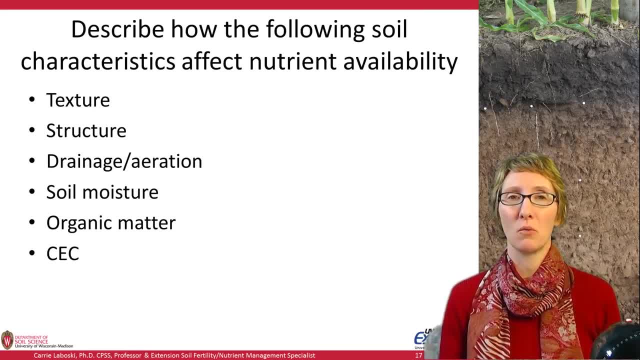 on all of these because some of this information is brought out in different ways As we're going through the other videos with focusing on some of the nutrients and other concepts. But keep in mind: how does texture affect nutrient availability? What about structure? And maybe in structure? 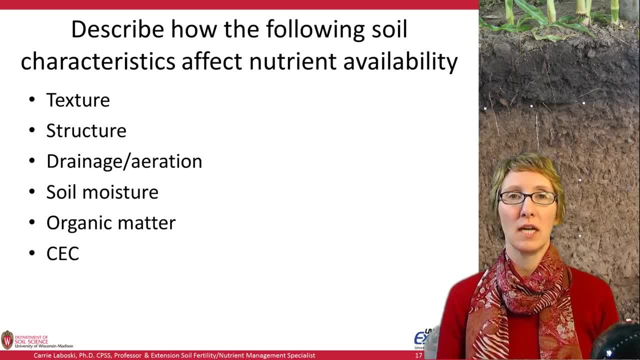 I'd throw compaction in there, because that's sort of a lack of structure. What about drainage and aeration? How does that influence particularly nitrogen? Soil, moisture, organic matter, cation exchange. they all interact together to affect nutrient availability, And that's something you should be able to. 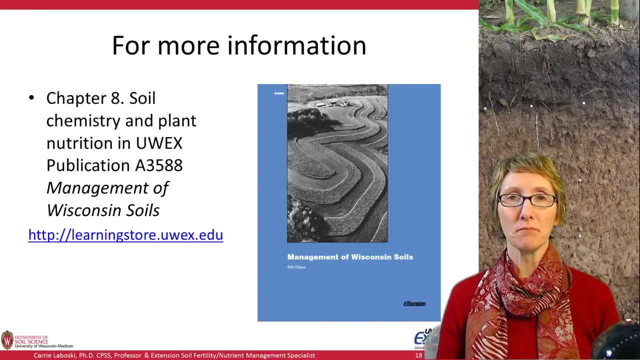 have an understanding of when you're taking the exam. So if you'd like more information, a good ready reference that you can find is in management of Wisconsin soils. chapter 8 is soil chemistry and plant nutrition, But of course there's many chapters in this. 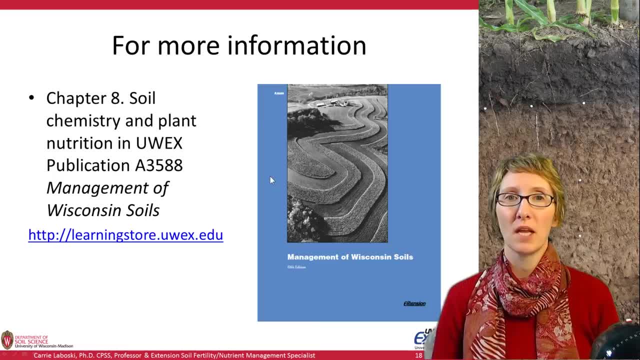 book that would be helpful to you. It's freely available for PDF download at the learning store, or you could also purchase the document. One caution I will put out is that this bulletin was last updated in, I believe, 2005.. And since that time we've had two updates. 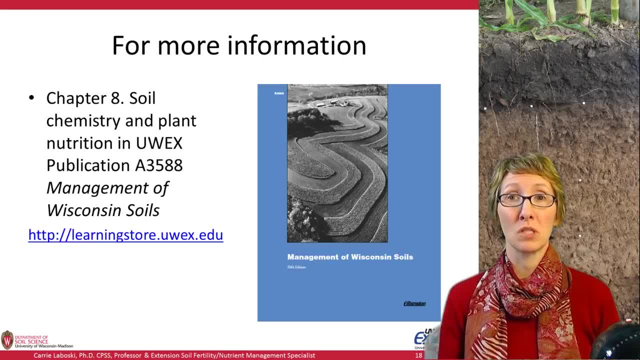 on our nutrient application guidelines bulletin. So when you get into some specifics of actual nutrient application rates, this booklet is outdated, but the many, many other concepts that are in this book are still perfectly fine. It's a good tool to use as you're. 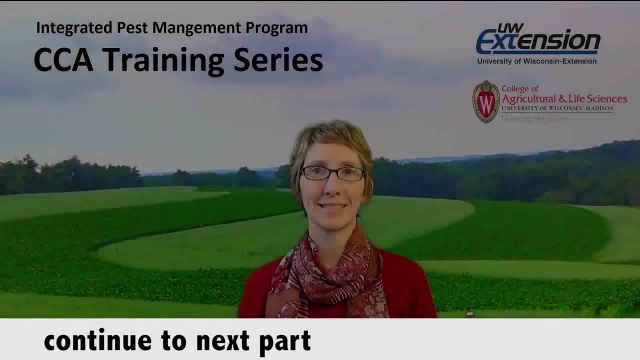 going through and studying Music, Music, Music.